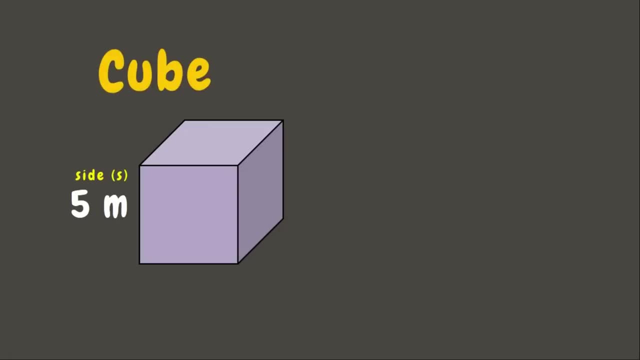 example, We have here a cube whose side measures 5 meters. To get a surface area of a cube, we are going to use the formula 6 times s squared, So that will be 6 times the square of the side, which is 5 meters. So that will be 5 meters times 5 meters. 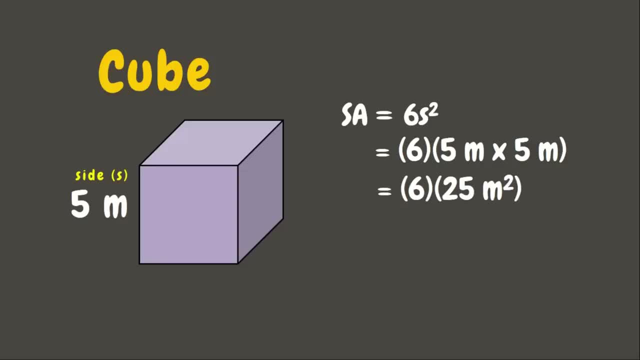 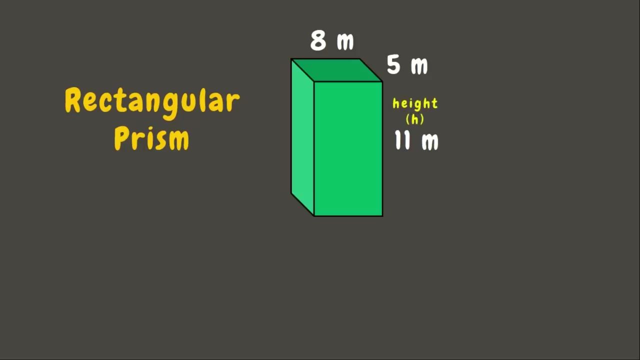 6 times 25 square meters is 150 square meters. Now, this is the surface area of this cube. Great job. Now, this time, we have a rectangular prism whose height measures 11 meters, length 8 meters and width 5 meters. Now to solve for the surface area of a rectangular prism. 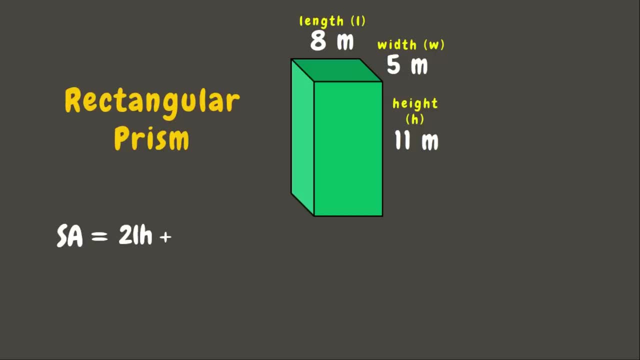 we are going to use the formula 2 times the length, times the height, Plus 2 times the length, times the width, Plus 2 times the height times the width. Let us try and solve First. we have 2 times the length, which is 8 meters, Times the height. 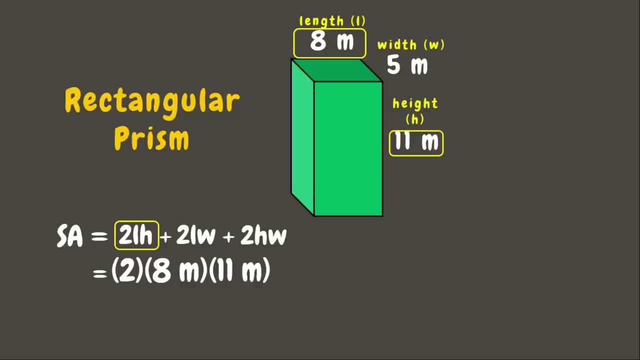 which is 11 meters, And if we solve for this one, we'll get 176 square meters. Next, let us multiply 2 times the length, which is 8 meters, times the width, which is 5 meters. If we solve for this one, we'll get 80 square meters. Next one: we have 2 times the height. 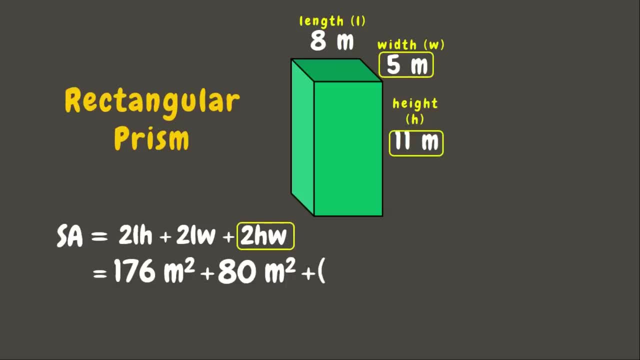 which is 11 meters, times the width, which is 5 meters, And that will be 110 square meters. Now let us add the 3 areas, That will be 366 square meters. Now, this is the surface area for our rectangular prism. Awesome, We have here a triangular prism whose 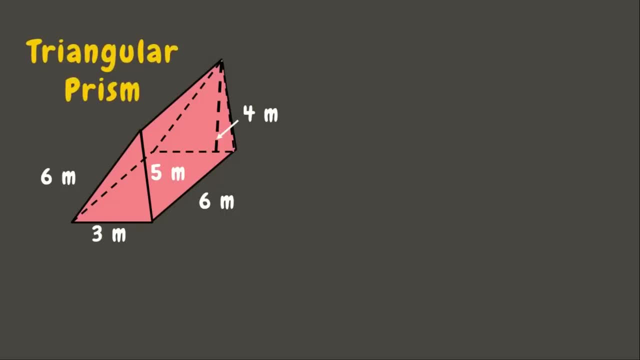 base are triangles And we can see that it has 3 sides, which is 6 meters, 5 meters and 3 meters. The length here would be 6 meters, while the height would be 4 meters. Now let us try and solve. 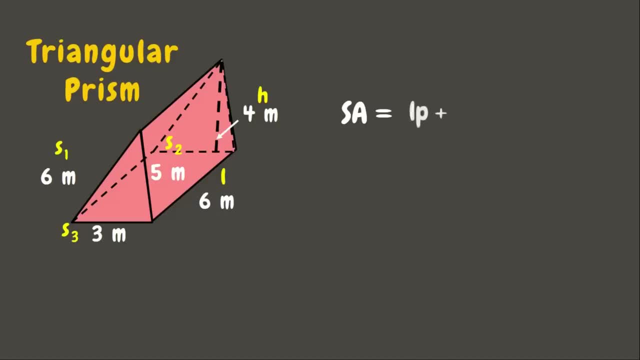 The formula for the surface area of a triangular prism would be the length times the perimeter of the base, which is a triangle, plus base times the height. First let us get the length, which is 6 meters times the perimeter of our triangle, which is the sum of its side. so that would be 6 meters plus 3 meters plus 5 meters, and that 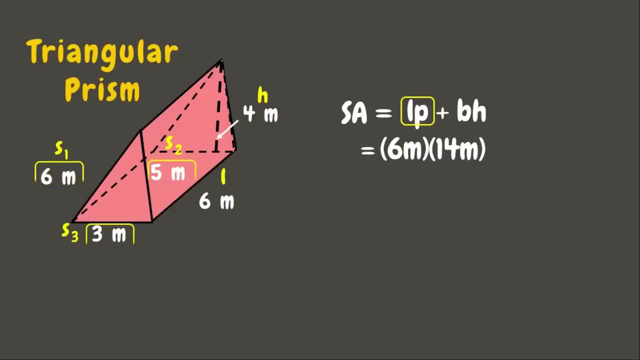 is 14 meters. Next we have base times, the height. Here the base is 3 meters times the height of the triangle, which is 4 meters. Now let us solve: 6 meters times 14 meters is 84 square meters, Plus 3 meters times 4 meters, which is 12 square meters. 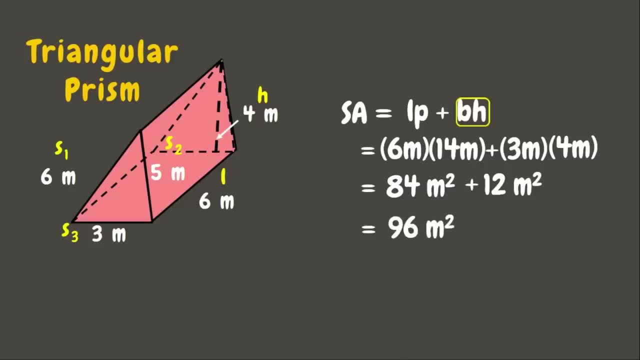 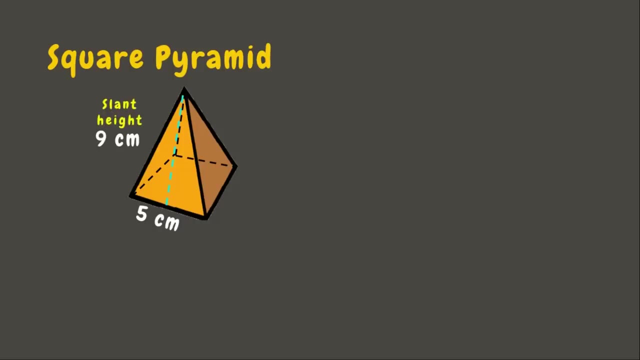 Now let us add the two areas, we'll get 96 square meters. Now, that is the surface area of this triangular prism. Awesome. Now let's go and have another one. This time we have a square pyramid whose slant height measures 9 centimeters, while the side 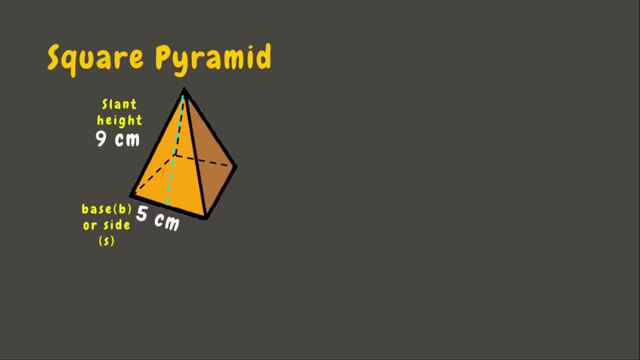 of its base, or the base of the triangle measures 5 centimeters. To solve for its surface area, we are going to use the formula 2 times the base times the height of the triangle plus s squared First, we have 2 times the base of the triangle, which is 5 centimeters times the height, which 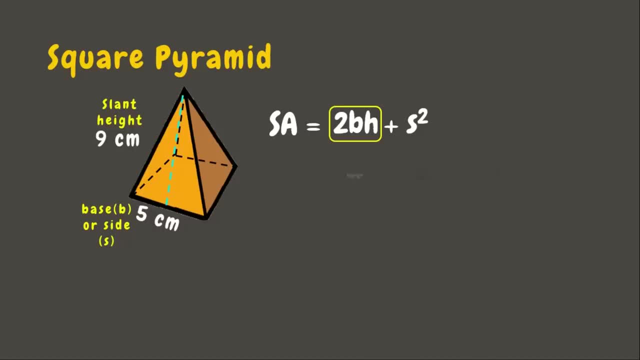 is 9 centimeters, and that is 90 square centimeters plus the square of the side of the base, which is 5 centimeters. So that will be 5 centimeters times 5 centimeters, And that is 25 square centimeters. 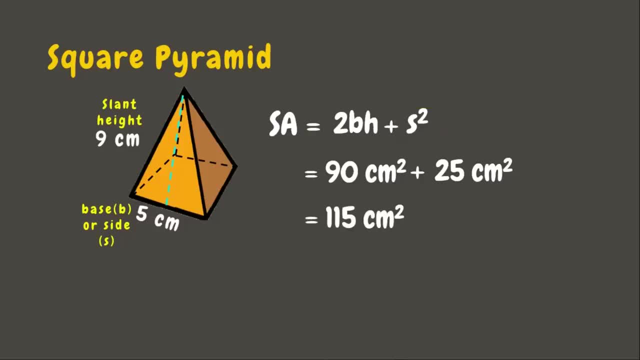 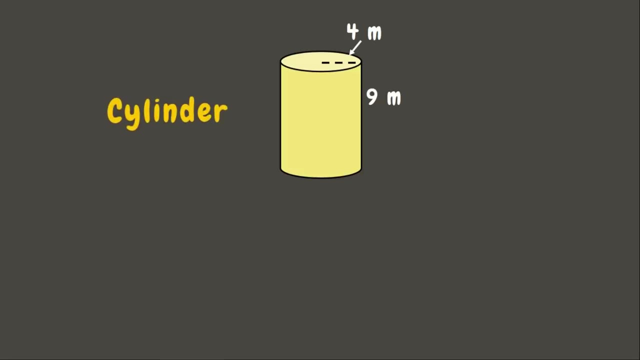 Let us add the two areas, we'll get 115 square centimeters. Now, this is the surface area of our square pyramid. Great job. Now let's have another figure. This time we have a cylinder. Our cylinder has the radius of 4 meters. 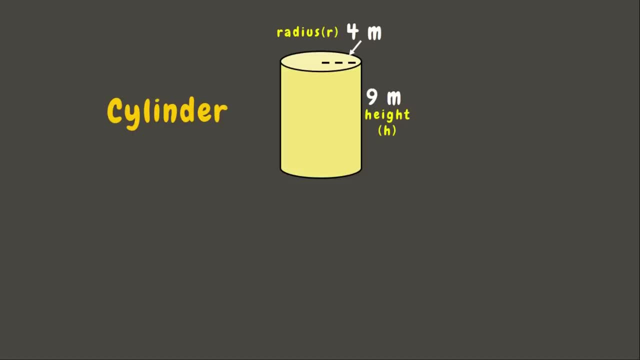 And the height of 9 meters. To get the surface area of a cylinder we are going to use the formula 2 pi r h plus 2 pi r squared First, let's have 2 pi r h. That will be 2 times the value of the pi, which is 3.14 times the radius, which is 4 meters. 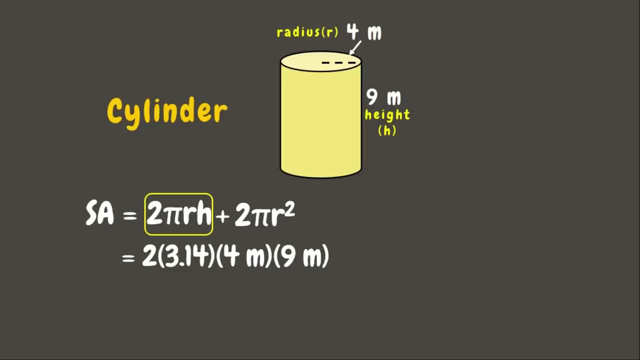 times the height, which is 9 meters. If we solve for this one, The answer would be 226.08 square meters. Next, we have 2 pi r squared, So that will be 2 times the value of the pi, which is 3.14 times the square of the radius. 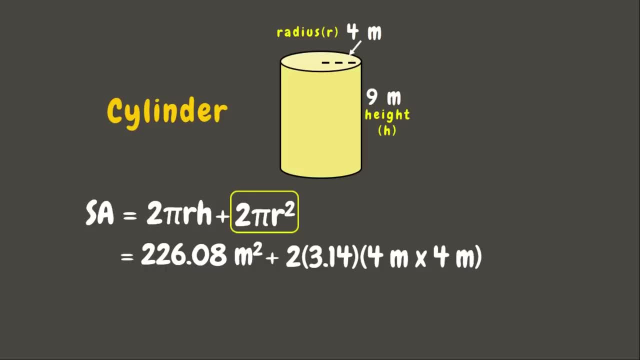 which is 4 meters. So that will be 4 meters times 4 meters. If we solve for this one, The answer would be 152.08 square meters, So that will be 2 pi r squared: 348 square meters. now let us add two areas. the answer is 326, point 56 square. 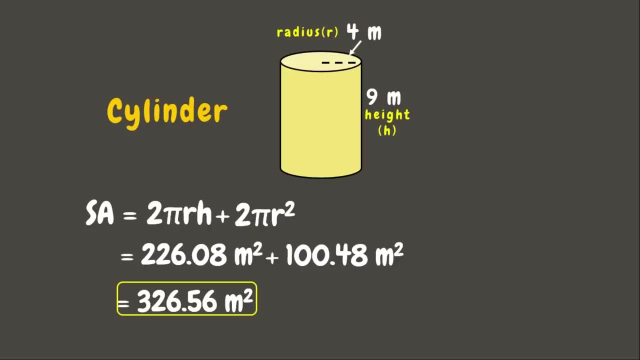 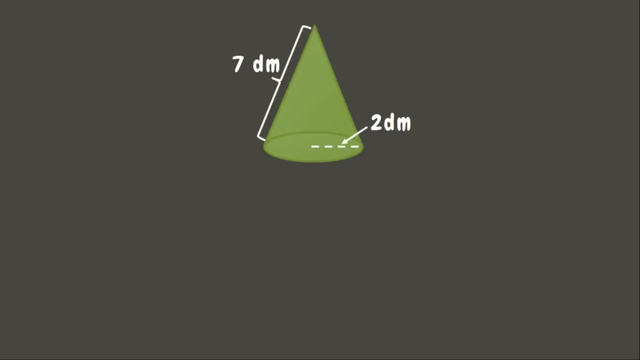 meters. now this is the surface area of our cylinder. wonderful, now let's take a look at another example. we have here a cone whose slant height measures 7 decimeters and their ranges 2 decimeters, the sole. for the surface area of a cone we are going to use the formula PI RS plus PI R squared. first let us solve PI. 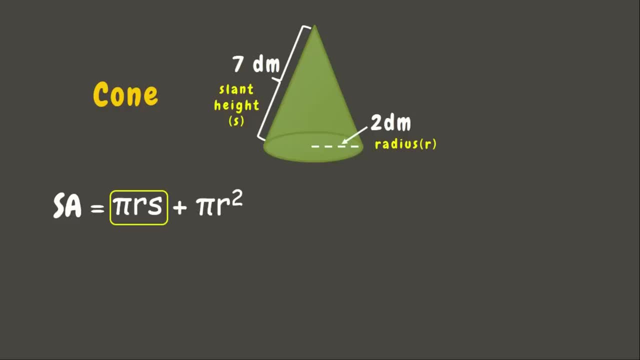 RS, that will be the value of PI, which is 3.14 times their ranges, which is 2 decimeters times the slant height, which is 7 decimeters, if we multiply it, as the answer would be forty three point ninety six square decimeters. 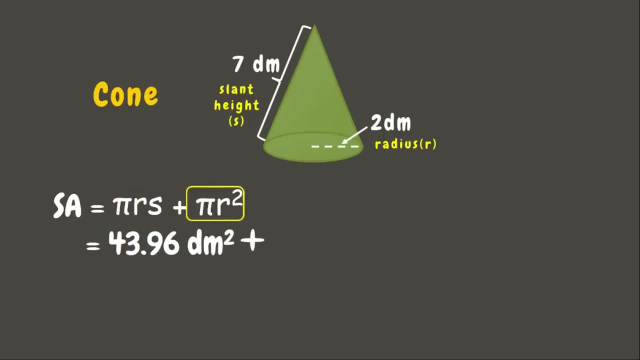 next we have PI R squared again, the value of our PI would be 3.14 times the square of our ranges. so that will be 2 decimeters times 2 decimeters, and that is 12 point 56 square decimeters. if we added two areas, the answer would be fifty.